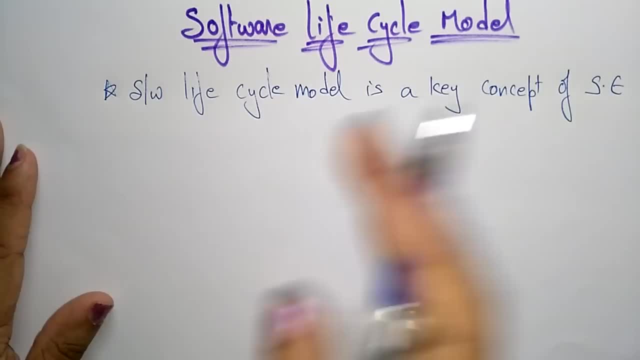 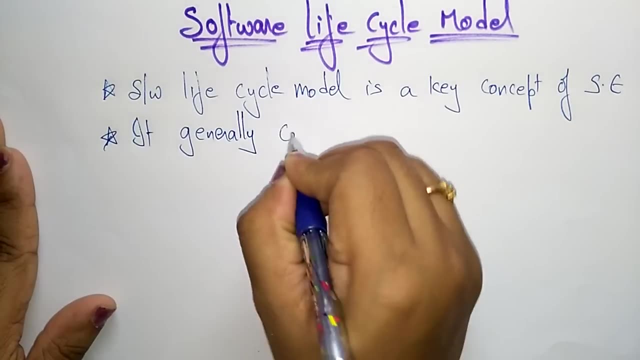 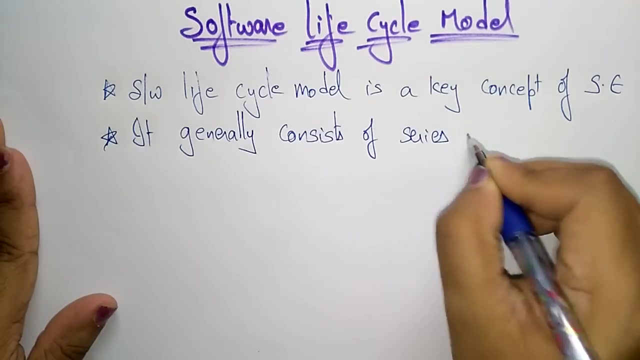 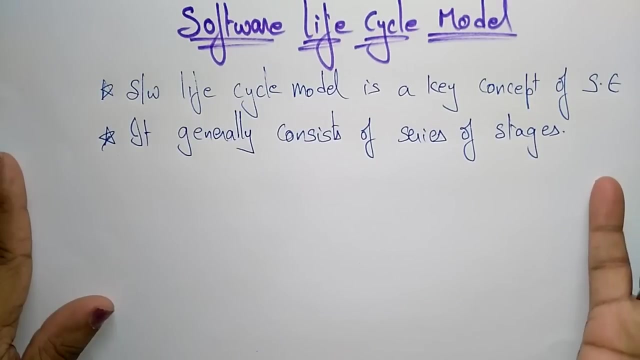 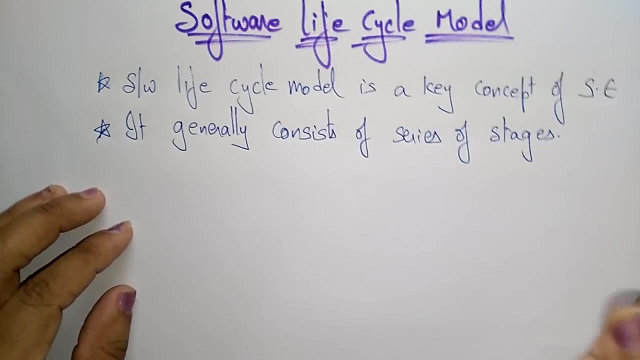 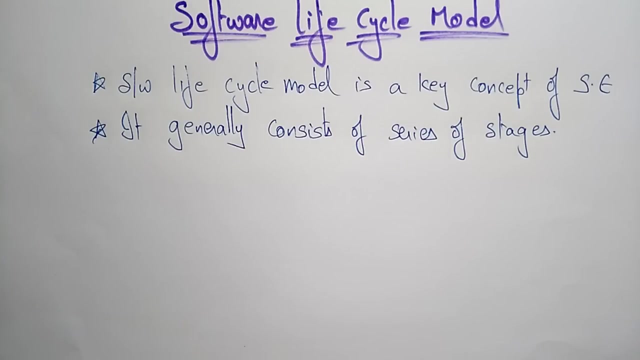 What do you mean by this life cycle? So it is generally consists of series of stages. So life cycle means you will come across series of stages. So in our life also we are having the series means at the starting I am a child, Next it's grown up, adult, Next it becomes woman. means this changes kid to child, child to adult. So like that, the cycle was changing, My life cycle was changing. So in the same way the software is having. also it's consists of series of stages. If you want to develop one thing, okay, you have to follow some steps that you call it as a software engineering. If I want to become a good person- means first I had. if I want to become a graduate, or if I want to become a graduate, I have to follow some steps. 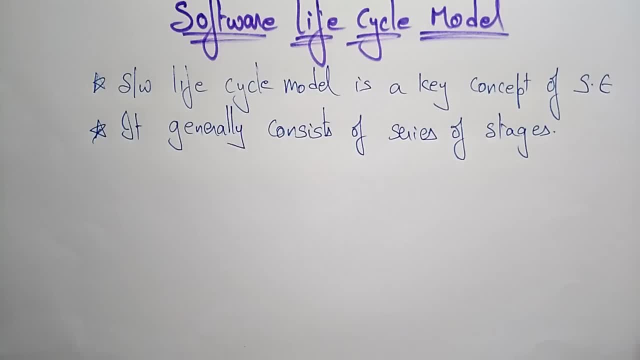 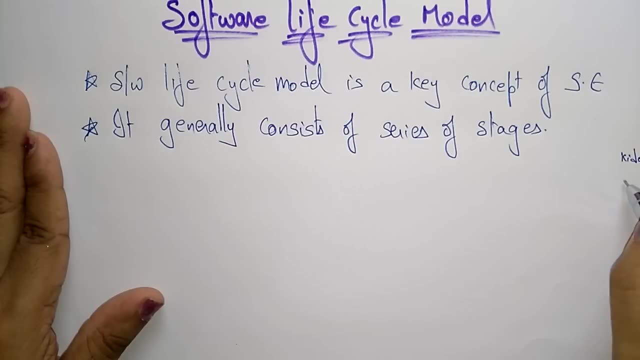 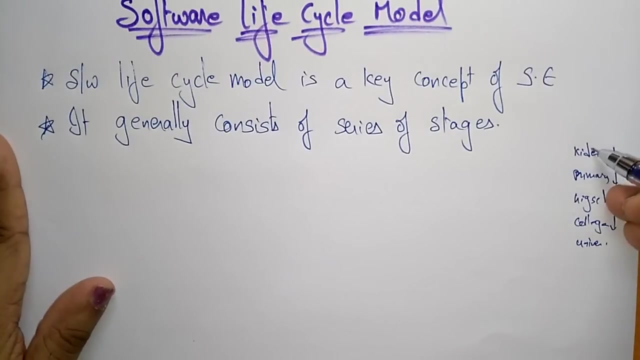 If I want to become a graduate, what I have to do? first I have to join, means when I'm in starting stage. first I have to join in the kindergarten, Next this school, primary school, next high school, college, Okay, university. So these are the stages that I'm changing from one one to another. first, kindergarten, primary, high school, college and university means my life cycle is changing. 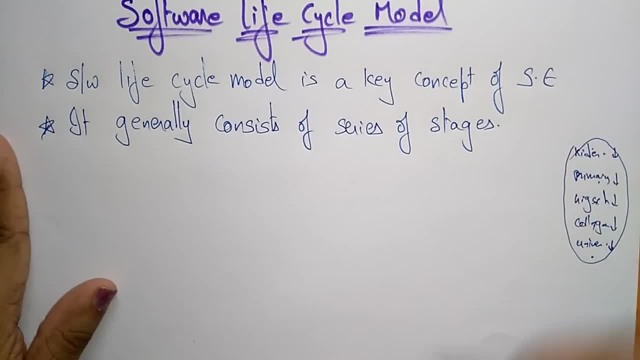 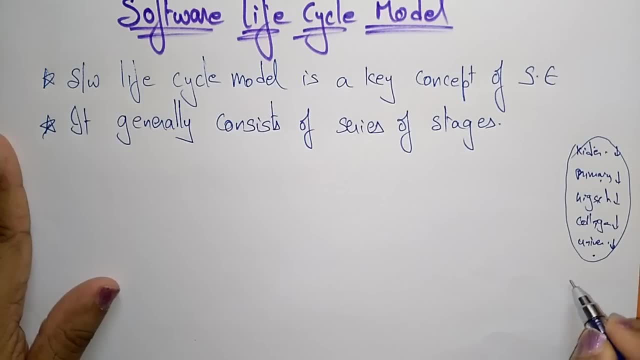 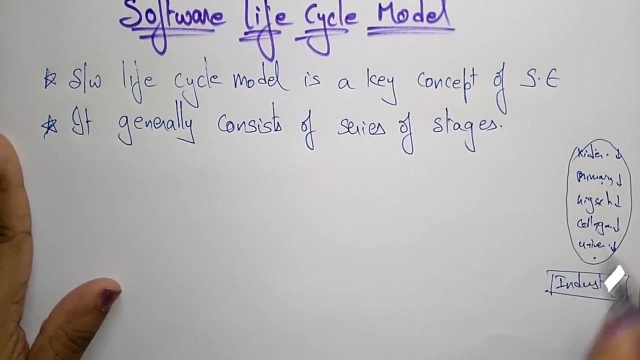 So if I didn't follow this rule, okay, I can't achieve my life means I can't enter into the suppose. if you want to join in a better industry, Okay, if you want to enter, if you want to join in an industry for a job, you want to need to complete in a sequence: First you have to complete kindergarten, next to primary, next high school, next college, next university, like that you have to be completed. So this is a systematic 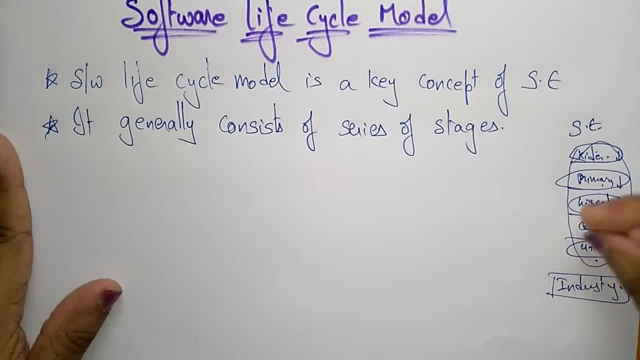 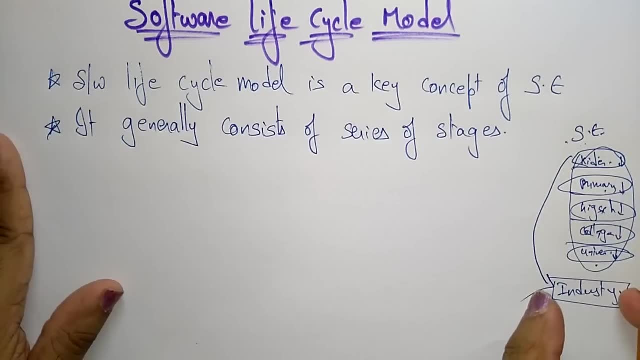 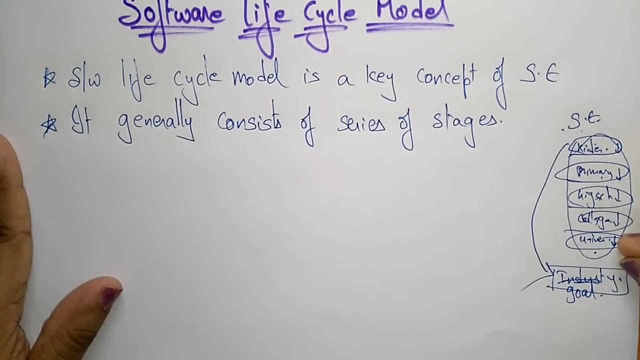 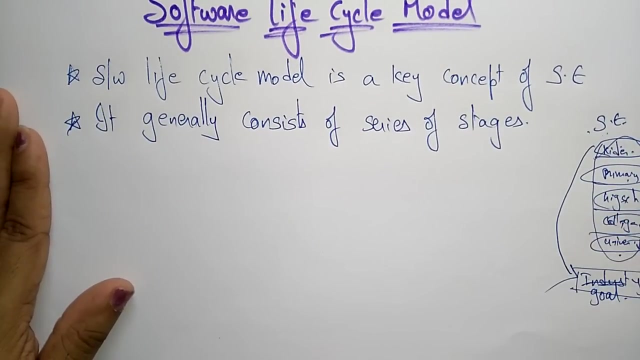 approach. This you call it as a software engineering. It is following a systematic approach and you'll, finally, you're reaching the person. The person is reaching to the his goal. Okay, whatever it may be, his goal is reaching his goal. So this you call it as a stages. in the same way, the software life cycle model is also consist of series of stages. So what are those stages? So first, it is should be analysis. 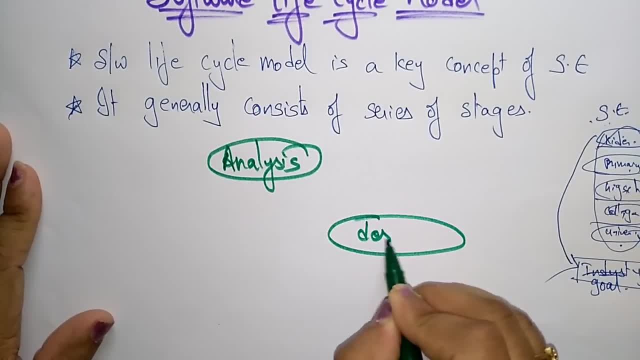 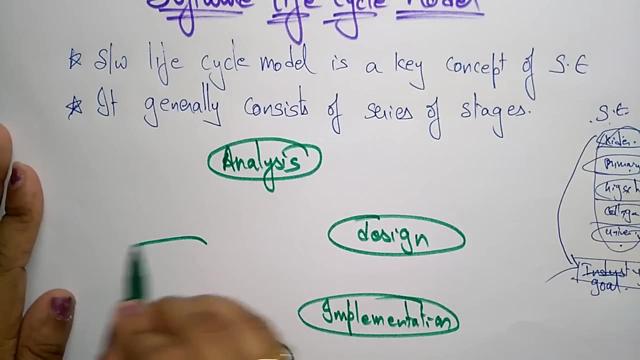 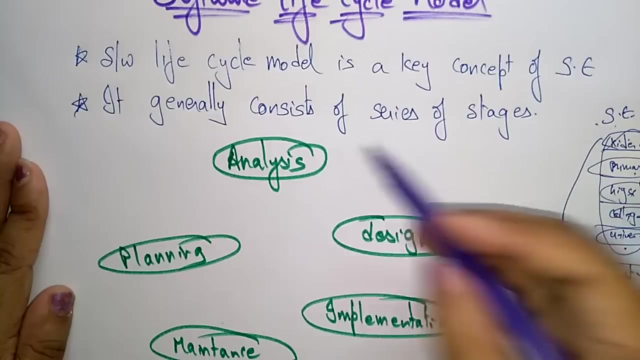 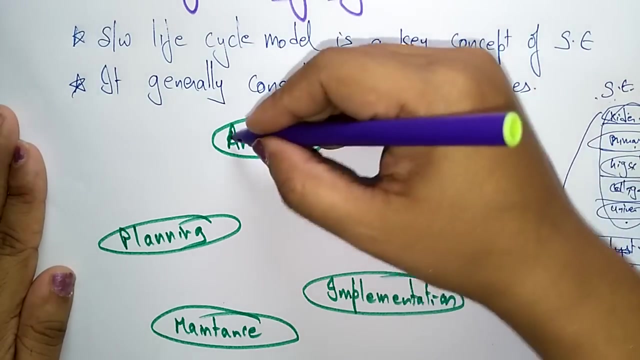 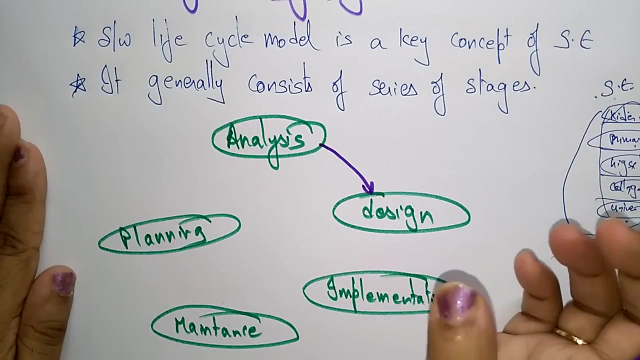 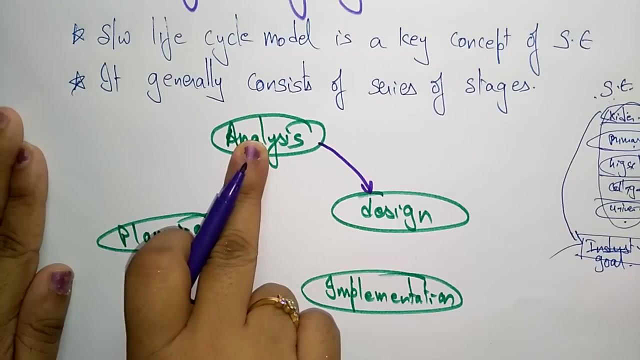 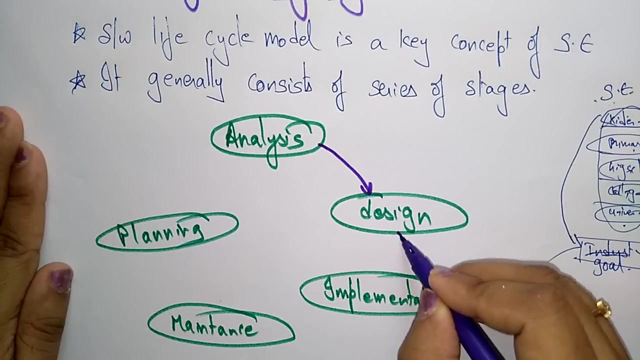 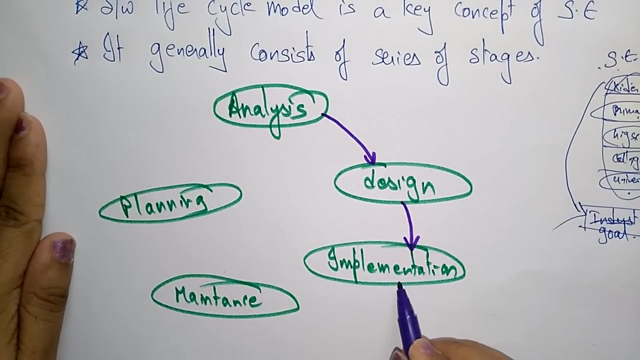 Analysis, next design, next implementation, maintenance planning. So these are the different stages in the life cycle model. First, whatever the problem you have taken, that should be analyzed. First you have to analyze. after analyzing the problem You have, you try to design that problem in a diagrammatic way so that you can understand rather than writing the code. If you represent in the form of diagrams, it will be easy for the persons to understand the topic. So first, analyze the topic, After that you have to design. If you get one view, you can design the product. Next, after designing, you can implement the product by using the code, by using testing everything. So after that you have to design. 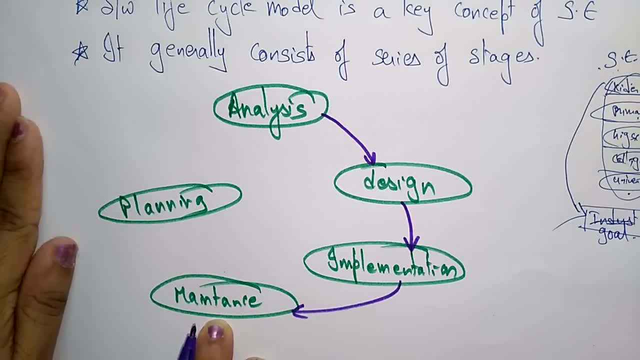 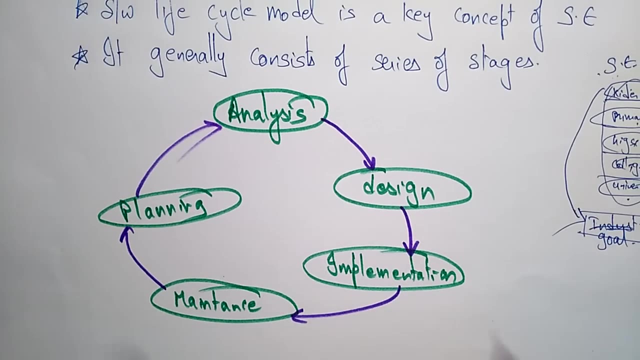 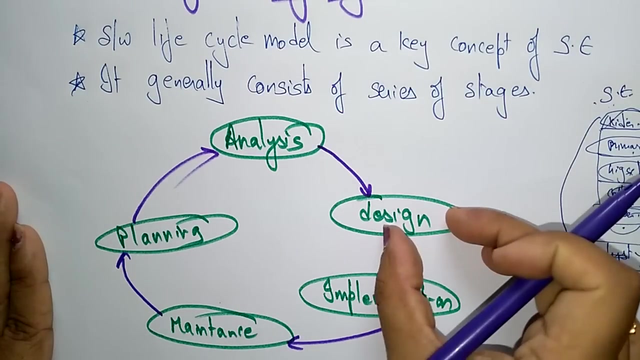 You have to maintain the product means whenever you deliver that product or anything. problem to a person means the solution that has to be maintenance. Next, you have to plan that And next analysis. Again, you can take another and just analysis. So this is a life cycle model. These are the different stages. Whenever one stage is completed, then only you can enter into next stage. next stage, like like. that means you have to follow a sequence of steps. 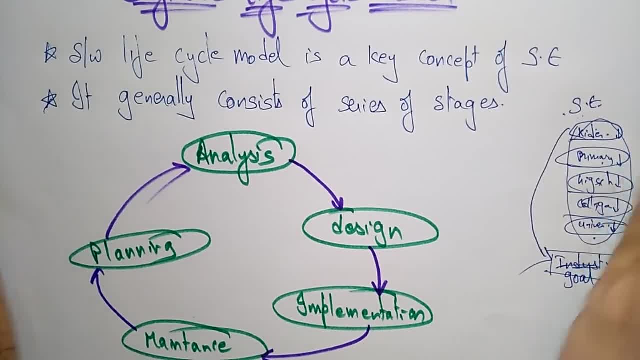 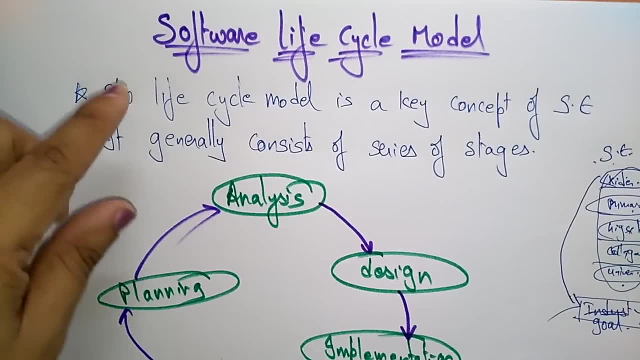 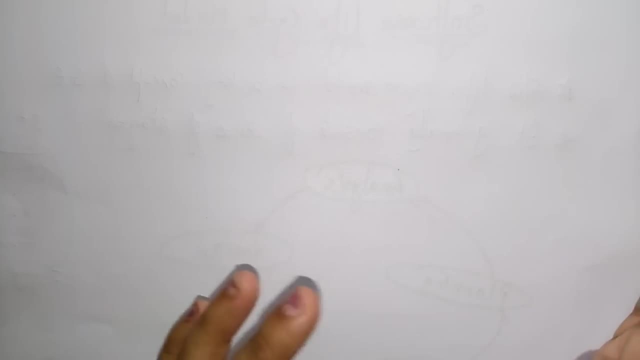 So, just like the example, what I have said now, Okay, so it generally consists of series of stages, So that you call it as a life cycle. Now coming to software life cycle model. So, even though life cycle is there, the life cycle model, software life cycle is there, Why we are going for different software life cycle models. Now let us see. So actually, this software life cycle is also called as software life cycle. 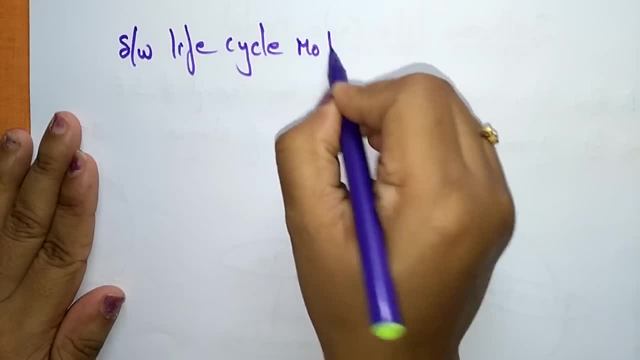 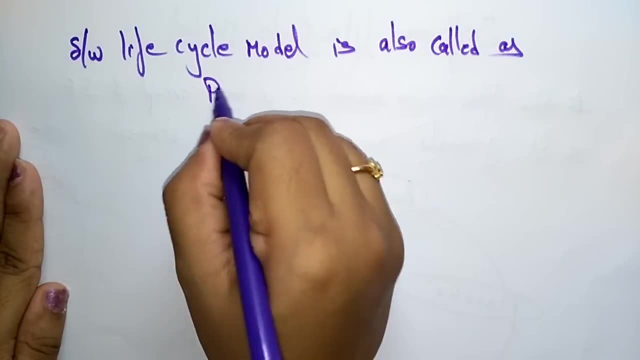 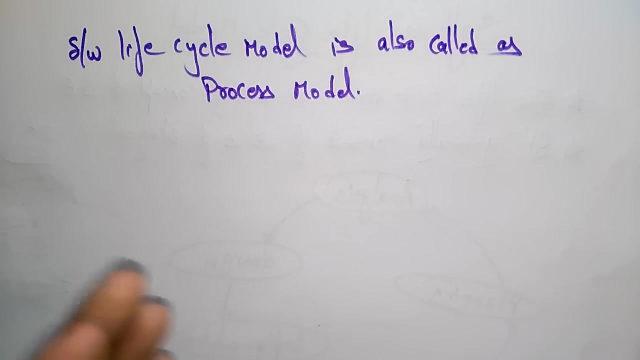 The software life cycle model is also called as process model, So both are the same process model. So this software life cycle model is a descriptive and diagrammatic representation of software life cycle. The definition for this is: the software life cycle model is a. 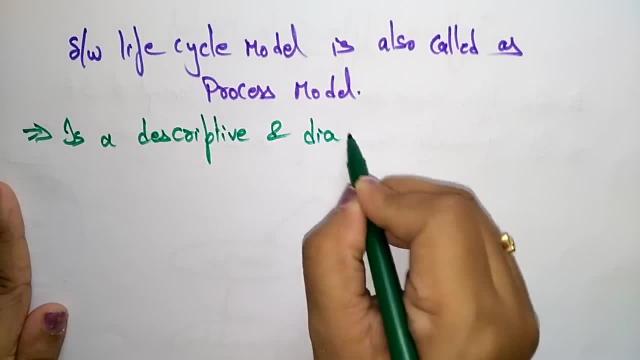 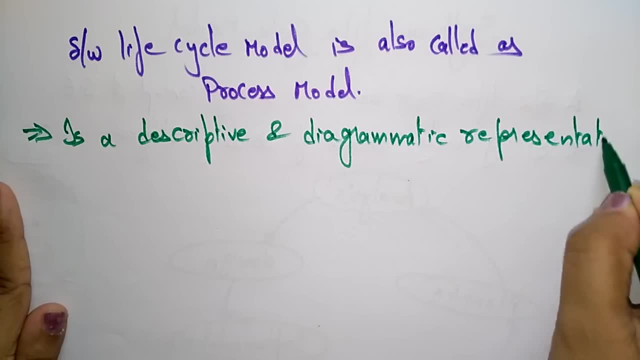 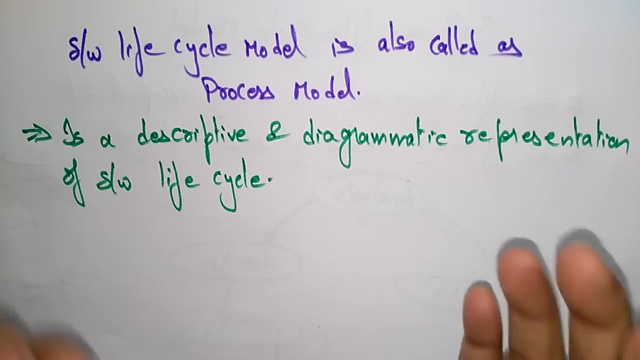 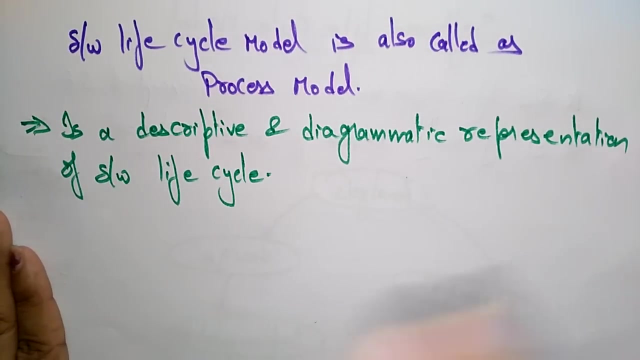 and diagrammatic representation of software life cycle that you call it a software life cycle model. so actually the software subject engineering is- you have to write your own. if you know the concept, you can write your own, but some definitions you have to write exactly like that. a software life cycle model is a descriptive and diagrammatic representation of software. 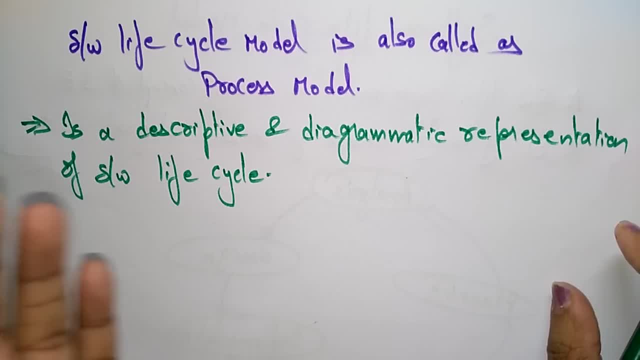 life cycle. so, actually, why we are using this software life cycle model. so, first of all, to overcome the software crisis, we are going. we are using the software engineering so, which is a systematic approach. so by using software engineering, you are going to develop a software product. so when you are developing a product, the development team must identify. 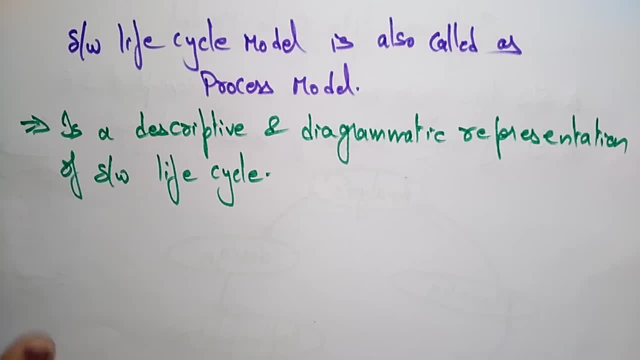 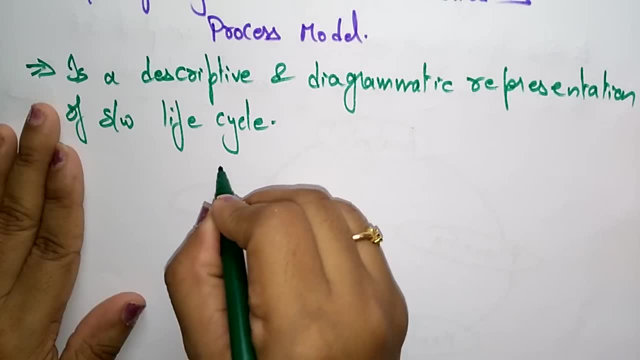 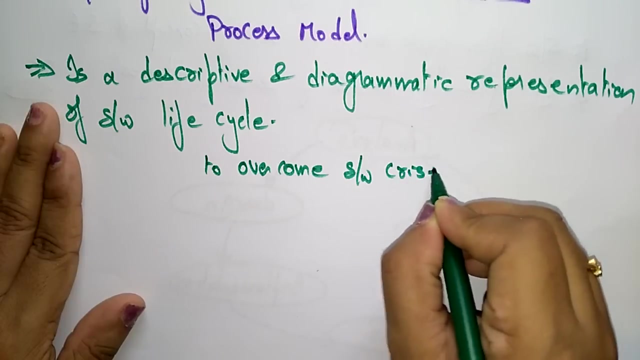 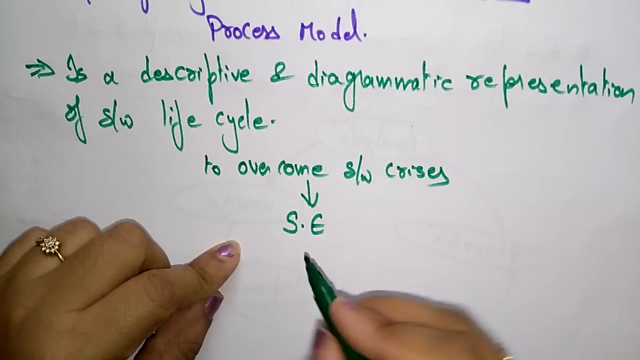 suitable lifecycle model for a particular project. let me explain now. so first, in the olden days, we are having so many software crisis. to overcome software crisis, software crisis, we are using software engineering. so, which is a systematic approach? so by using software engineering, we are going to develop a 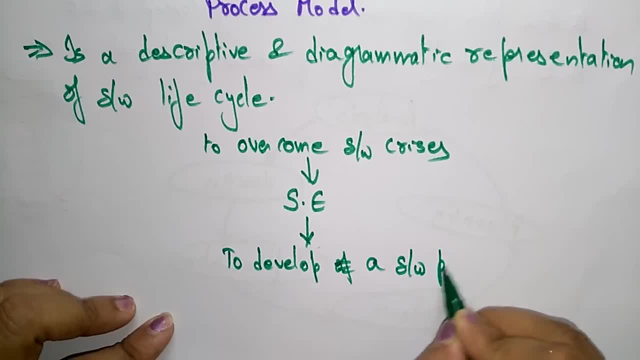 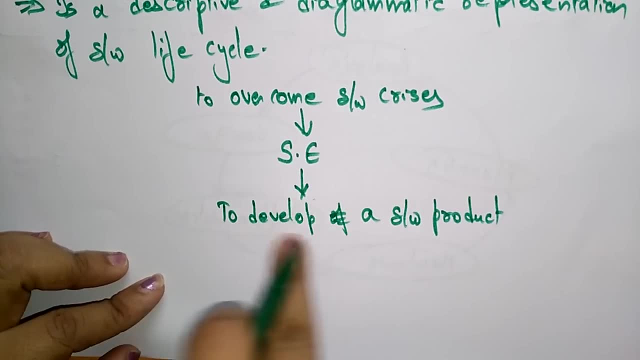 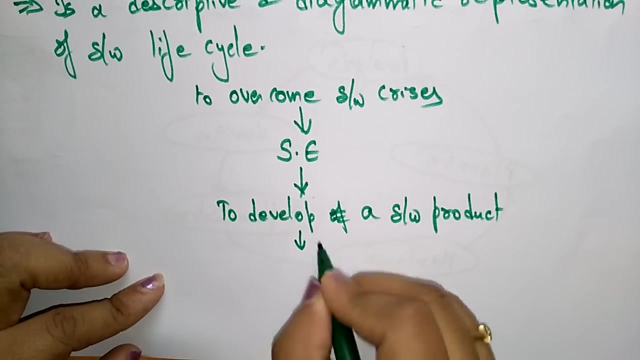 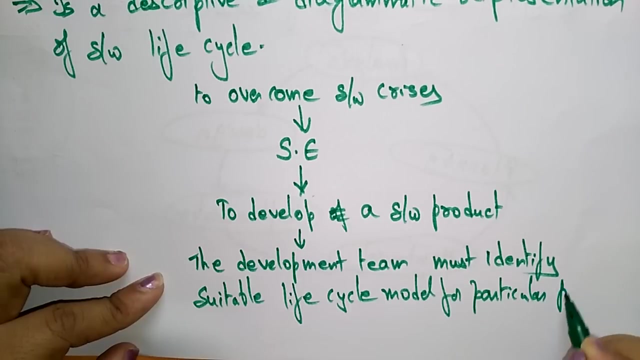 develop a software product. so to overcome software crisis, we are using software engine. the software engineering is used to develop a software product. so this developer, this software product, can be developed by a team. here the development team must identify suitable lifecycle model for particular project. so each project is having their own specification. so, based 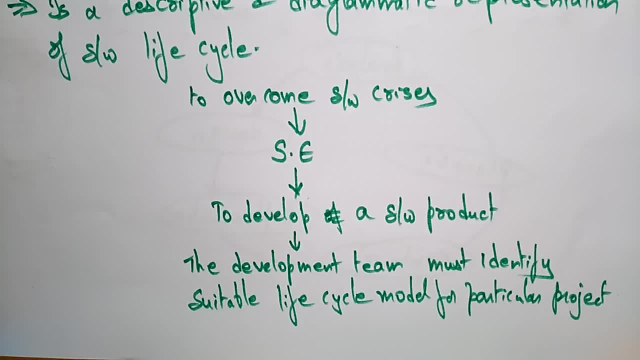 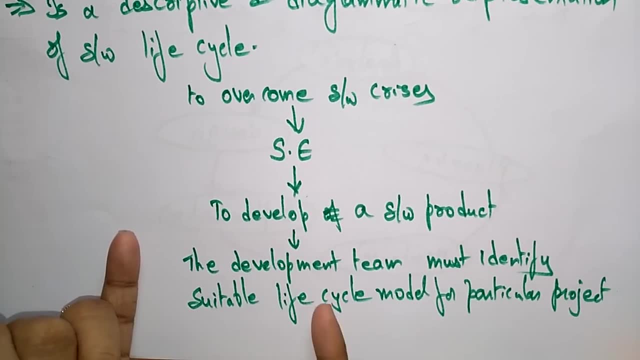 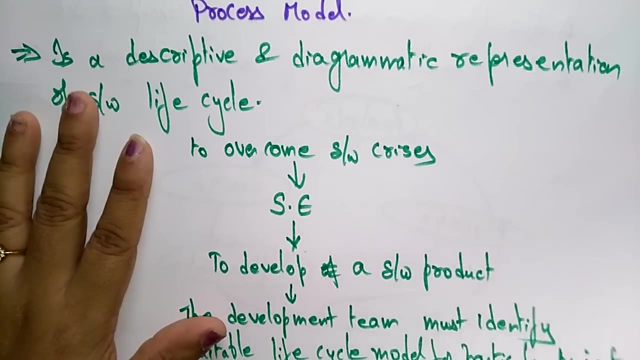 on the specification and based on the requirements and based on the time they are given. you are using different lifecycle models, so to develop any software product, the development team must identify suitable lifecycle model for that particular project, whatever they are doing. so this software lifecycle model defines entry and exit criteria for every phase. so analysis, phase design. 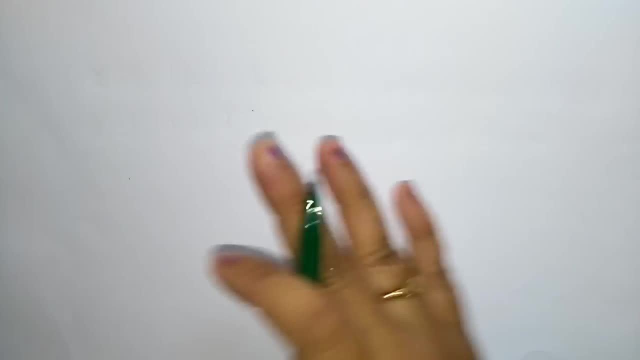 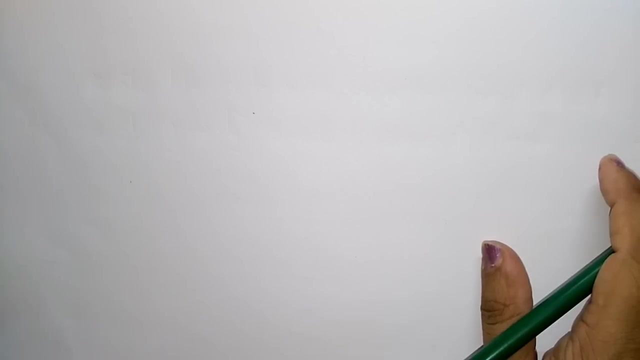 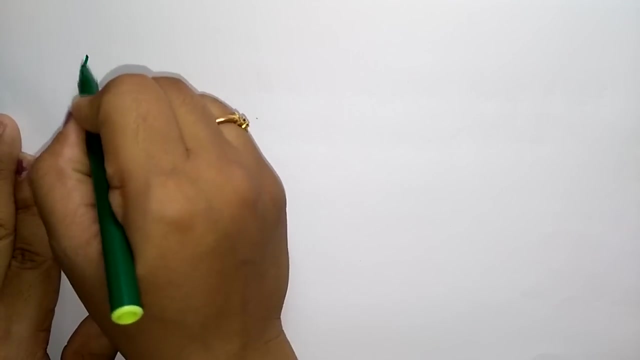 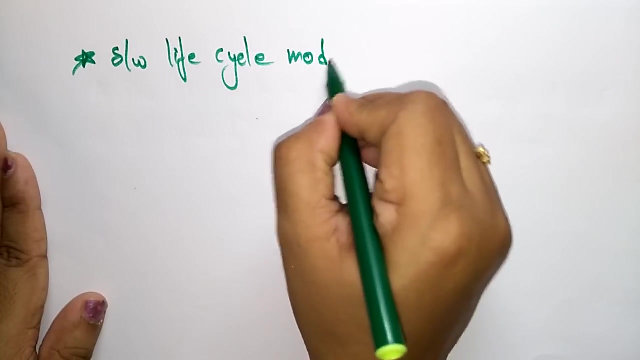 phase and implementation. for each and every phase there should be an entry and exit. so without software lifecycle model it becomes difficult for software product project manager to monitor the progress of project. so let me write the point so that you can know refer that software lifecycle model: define defines entry and. 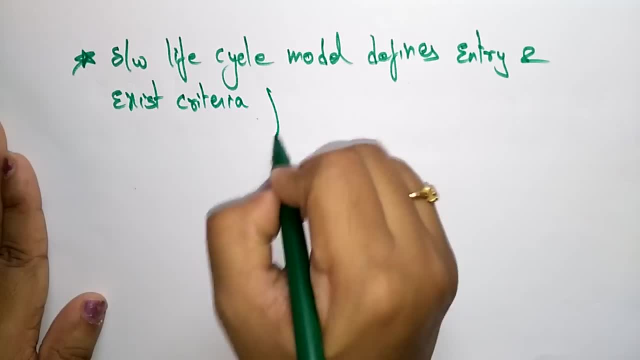 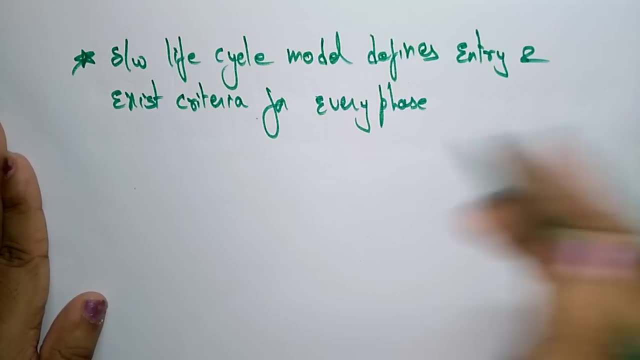 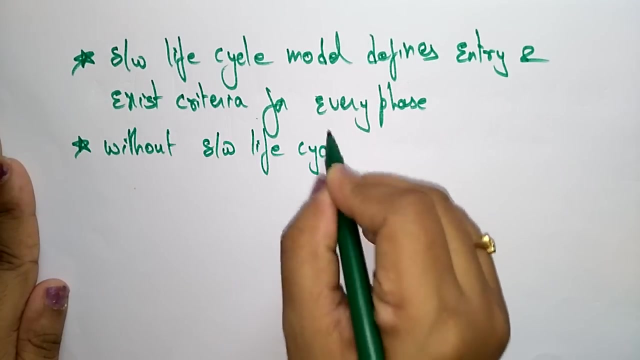 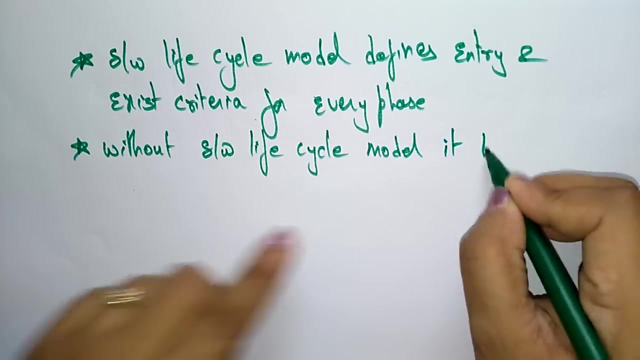 exist criteria for every phase. so whatever the phase there means that for every phase there should be an entry and an exit, and next, without- if you didn't use a software lifecycle model, means you are directly following the normal approach. so without software lifecycle model it becomes difficult for the product managers it becomes difficult. 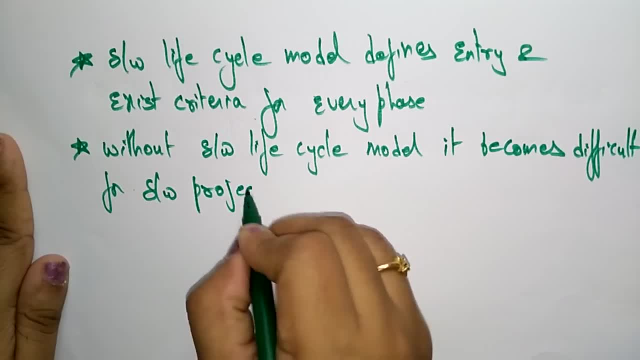 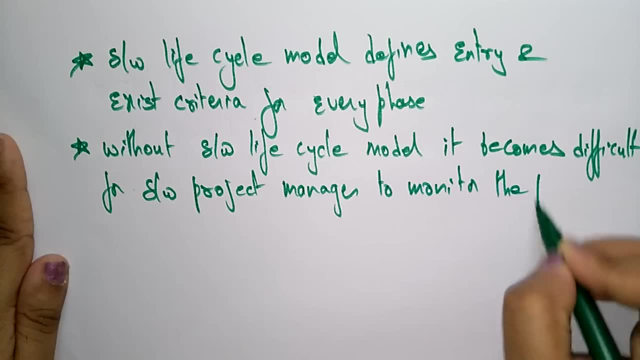 for software product managers, product or project manager to monitor the progress of project, because they they want to know in which stage their project is, should be there. so if you follow the systematic approach, if you they follow the software engineering techniques, then it will be easy for the project project manager uh for monitoring the project. 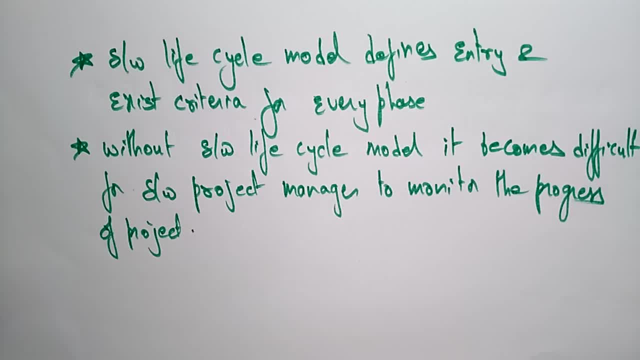 means in which stage. so after the completion of one stage only, the person has to enter into another stage. first they have to do analysis after analysis. if you get the one idea, then they go for the designing. okay, the designing is completely over. then they go for the implementation. like that they have to follow. 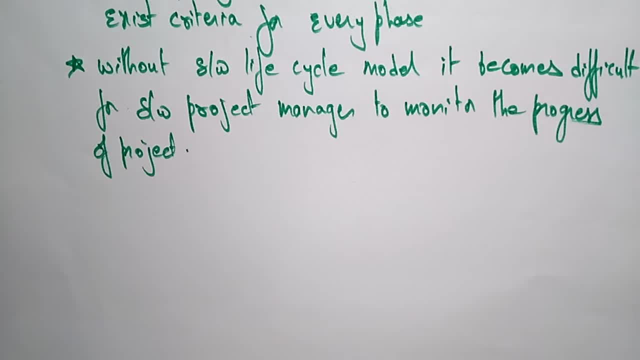 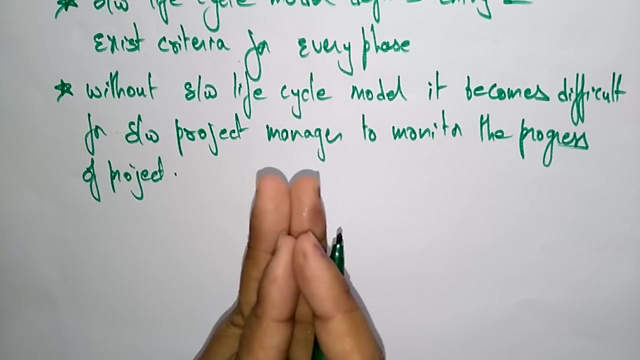 some systematic approach. so without using a particular model, the development of product would not be systematic and disciplined manner. so you have to follow systematic approach. so the one thing you have to be remember that when a software product is being developed by a team- suppose you are the team you are going to develop a software product- there must be clear understanding. 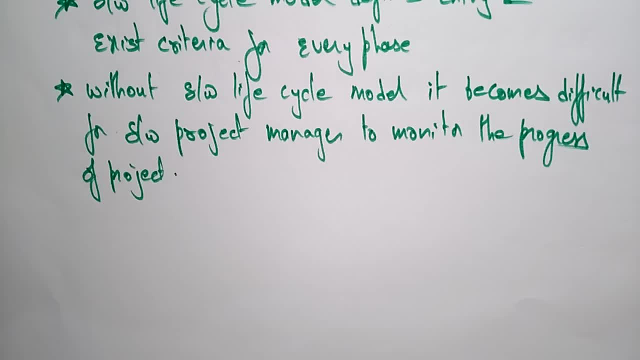 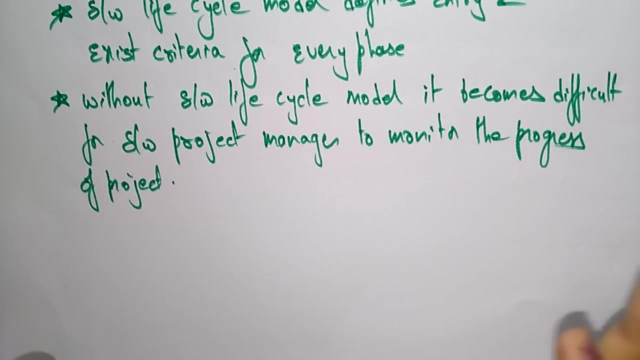 among team members about when and what to do. so, before you are developing a product, the team members must have a clear understanding among the team means about when and what to do. otherwise it would lead to a project failure. so this is a brief description about the software life cycle. now